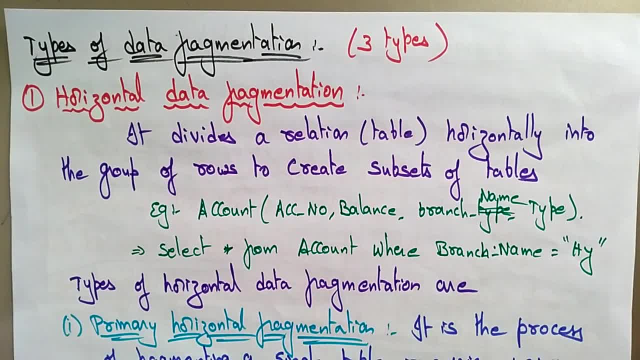 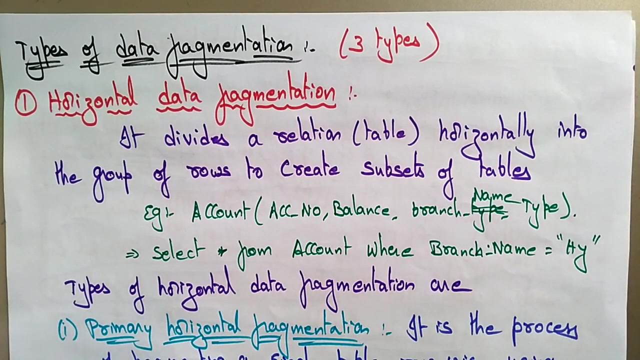 types of data fragmentation. so i said, after splitting the one database into several fragments, each fragment is stored in different locations. after that you are going to maintain the original database. means that is all the locations. fragmented data has to be reconstructed and you have to maintain that in a original database. that is the data. fragmentation means combining the data which 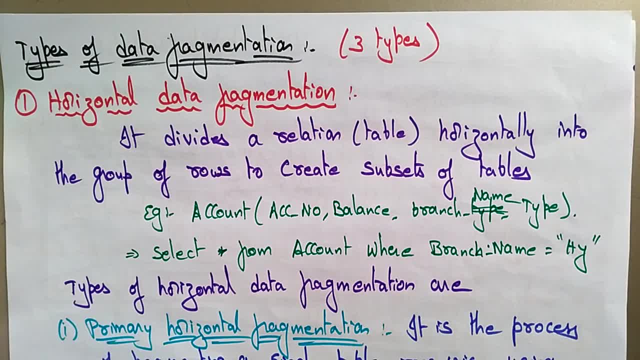 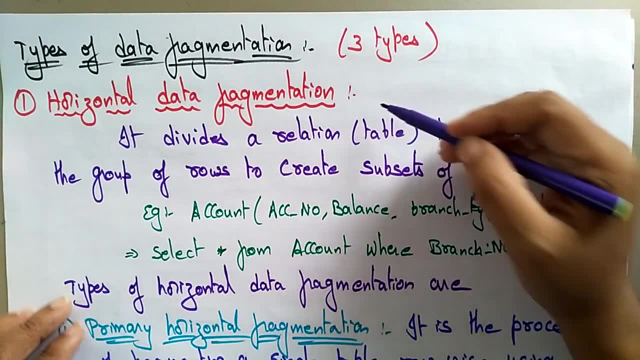 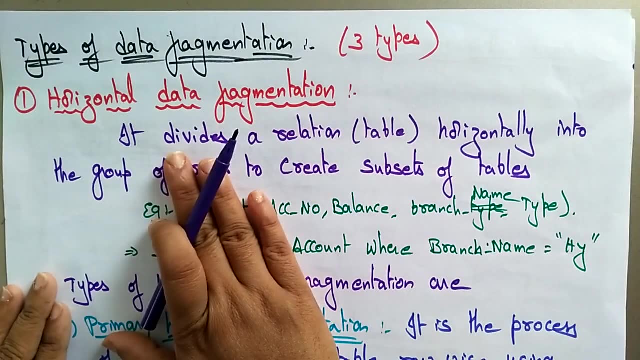 is present at different locations. reconstructing the data at different locations is the data fragmentation. there are three types of data fragmentation. now let's see one by one. the first one is a horizontal data fragmentation. so again, this horizontal is divided into different types. first let me explain you what is the horizontal data fragmentation- the name itself, 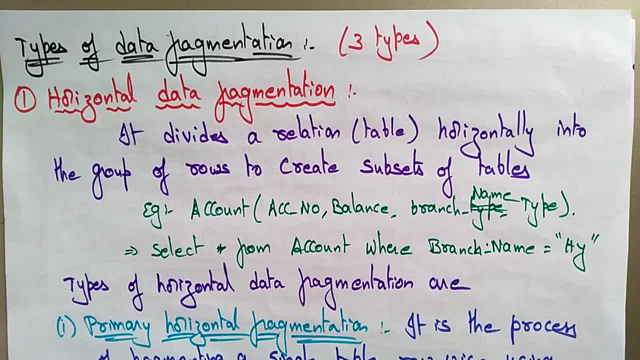 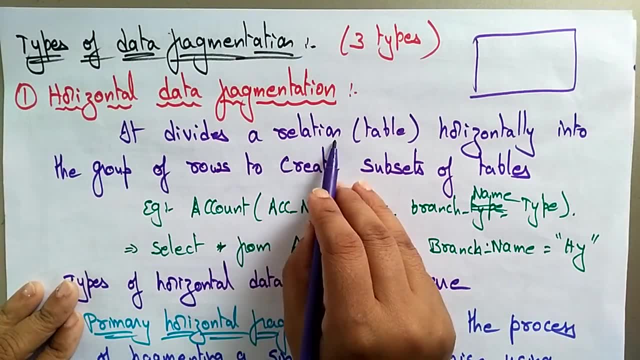 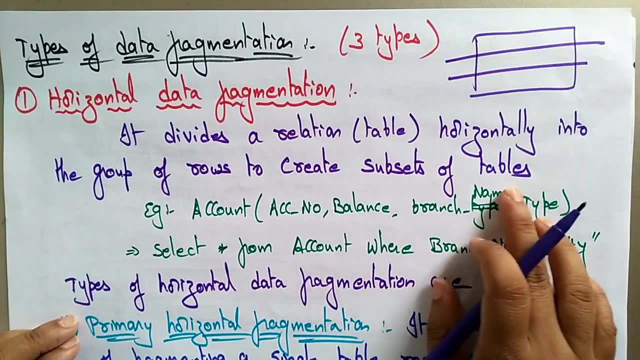 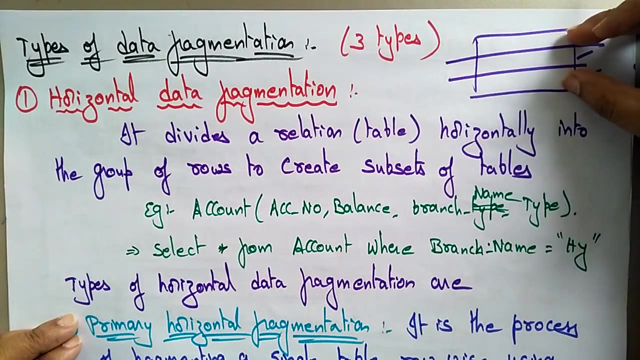 is saying that it horizontally. it divides the table horizontally into the groups. okay, if it. if you take a relational table, it divides a relational table horizontally, horizontally into a group of rows to create a subsets of tables. okay, so here you take it. this is one subset, this is another subset. so, like that, it dividing the complete database table into. 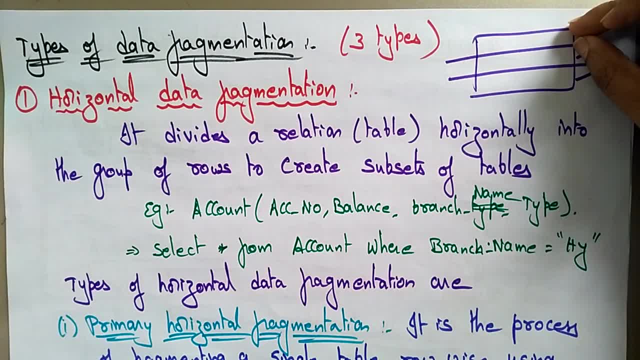 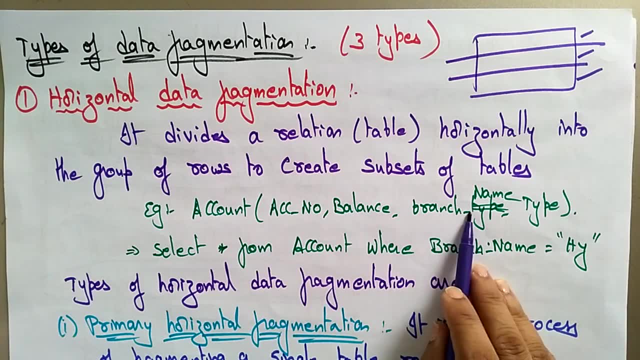 horizontal rows and it is grouping them to create a subset of tables. suppose, if you take an example, account is a table name. account number balance branch name and the type. okay, so here the account number balance branch name, type is there? select star from account where branch name is equal to header pattern. okay, only that. 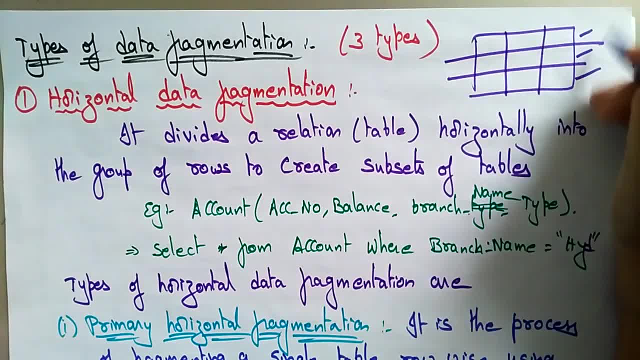 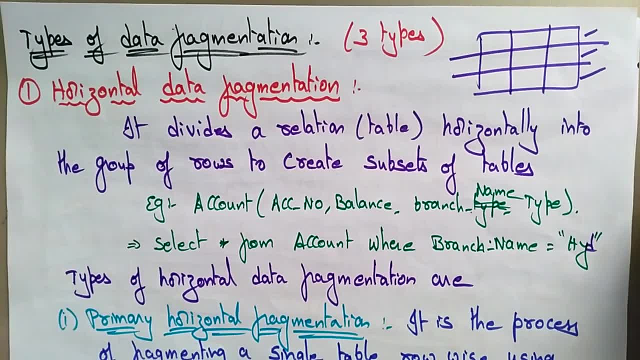 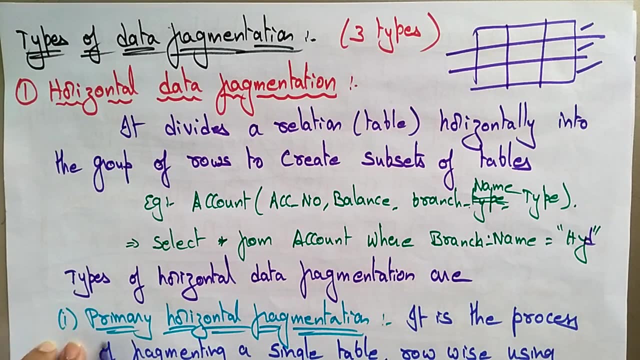 particular uh- horizontal row i'm going to be selected, only that particular horizontal row i am going to be selected. that is a horizontal data fragmentation. again, this horizontal data fragmentation are divided into different types. there are different types. first, if you take the primary horizontal fragmentation, it is a process of fragmentation, fragmenting a só. 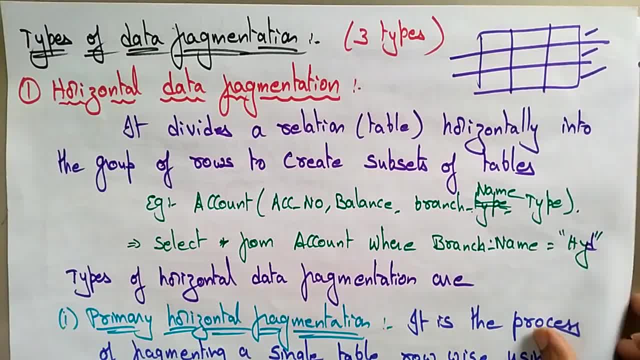 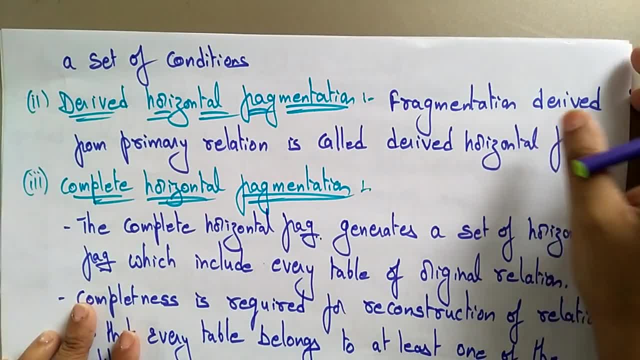 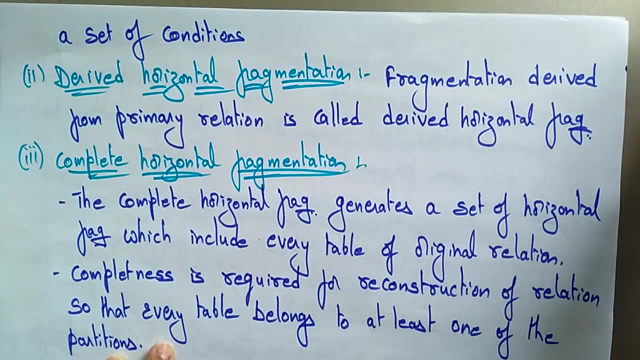 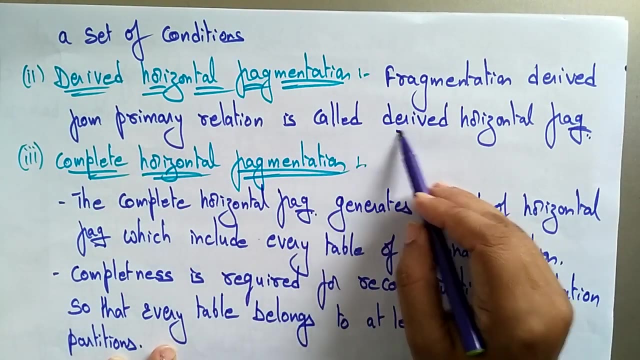 ого a á néo ána. single table that is a row wise, using using a set of conditions. and the second type of horizontal data fragmentation is derived horizontal fragmentation- the primary horizontal you have seen and the derived horizontal means the fragmentation is derived from primary relations- is called 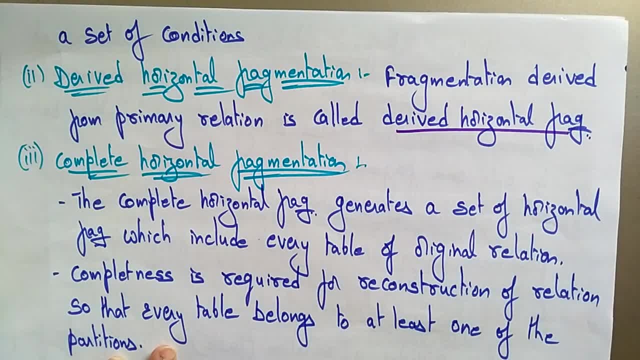 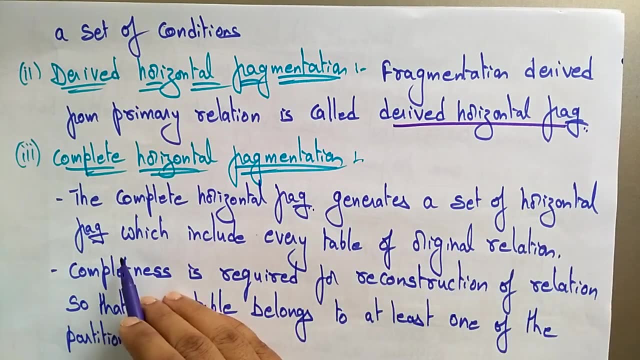 derived horizontal means it's just like a foreign. you are going to derive the fragmentation from primary relation that is derived. and another type of horizontal data fragment is complete horizontal fragmentation. the complete horizontal fragmentation generates a set of horizontal fragments which includes every table of original relation and its completeness is required for. 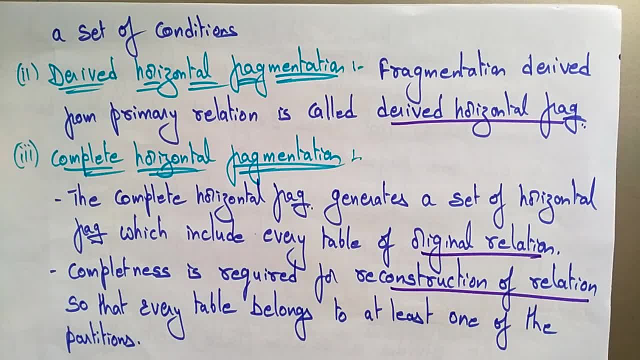 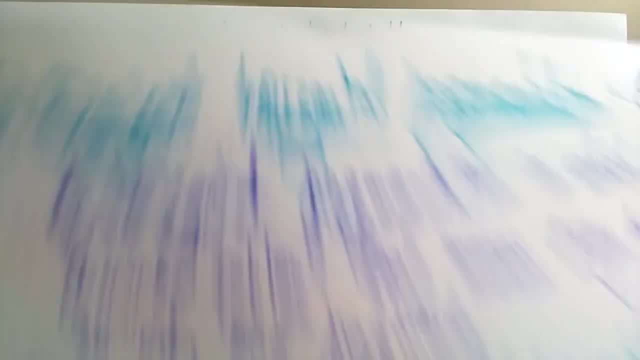 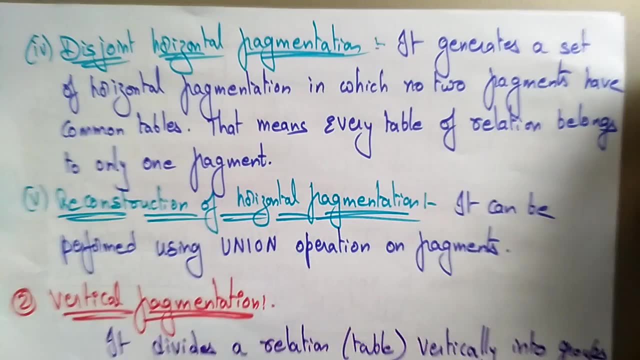 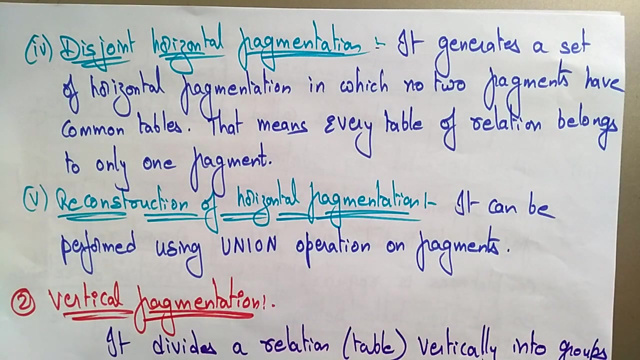 reconstruction of the relation so that every table belongs to at least one of the partitions. so the here the complete horizontal fragmentation. and another type of the horizontal is a disjoint horizontal. what this disjoint horizontal will do: it generates this complete. all concept is relating to the only. it's a group of rows because the table is divided. 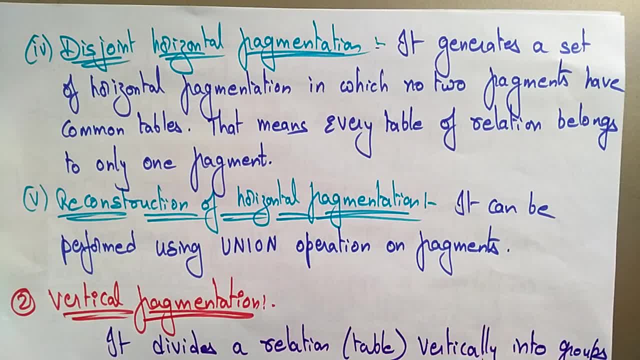 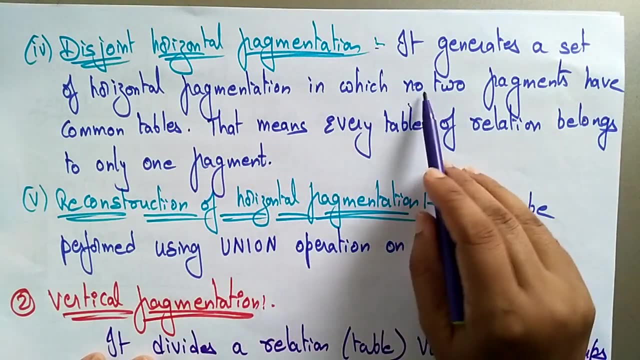 into horizontally into group of rows. we are performing the operations on that group of rows to create a subset of the tables. so further. these are all the different types of data fragmentation. that is a horizontal. next is a disjoint horizontal fragmentation. so this is a disjoint horizontal. uh aside, it generates a set of horizontal fragmentation in which no two fragments have. 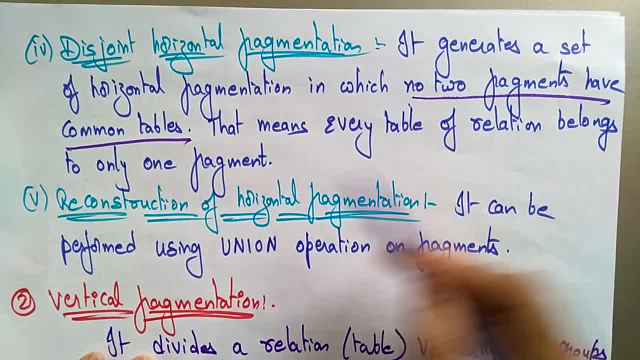 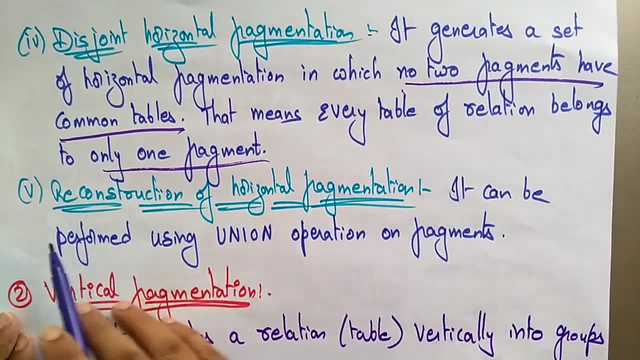 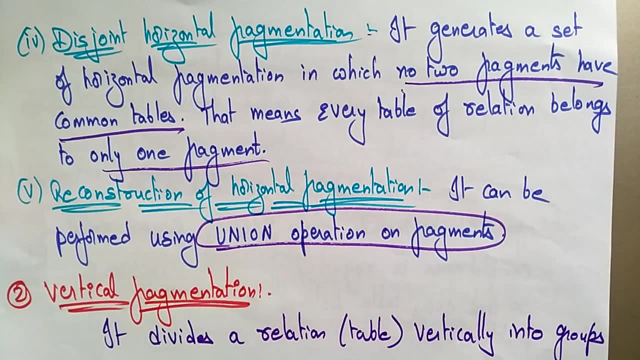 common tables. that means every table of relation belongs to only one fragment only. so that should be important. it is maintaining a unique relation, and next is a reconstruction of horizontal fragmentation. it can be performed by using union operation on fragments. so after completing of the fragmentation- uh, actually the data fragmentation itself is reconstruction. so how it is going? 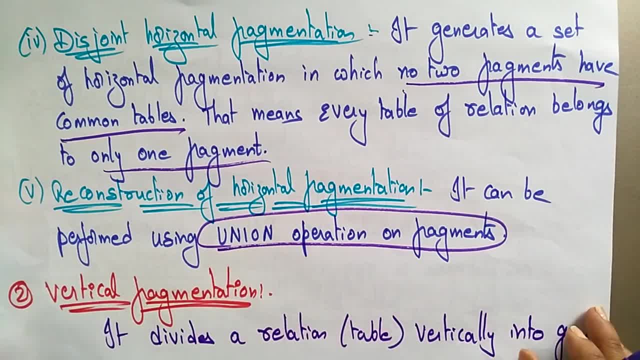 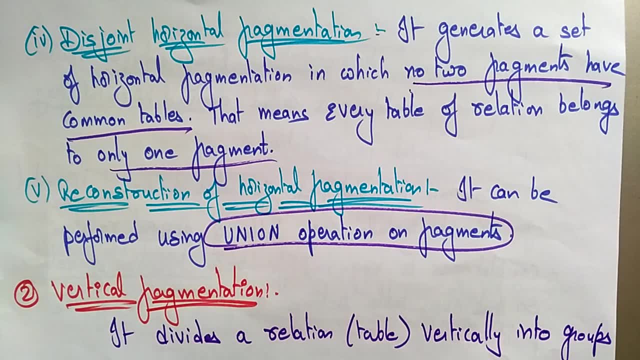 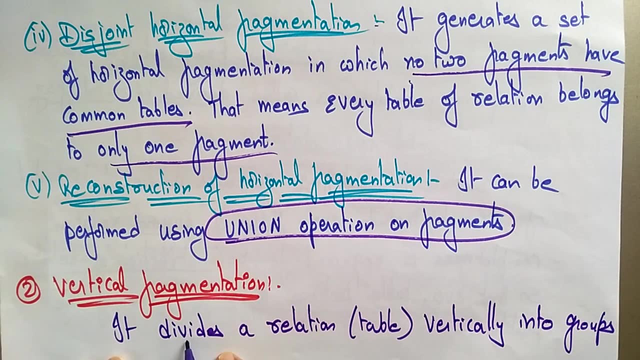 to reconstruct it by using the union operation. now coming to the next type of data fragmentation, that is, a vertical fragmentation. you have seen the horizontal and the next is a vertical. totally, there are three types of fragmentation: data fragmentation and the second one is a vertical, so horizontal. 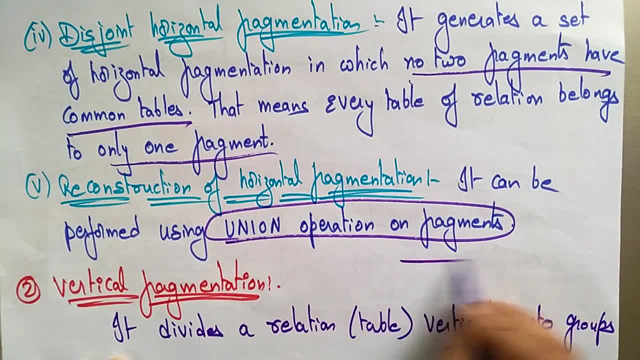 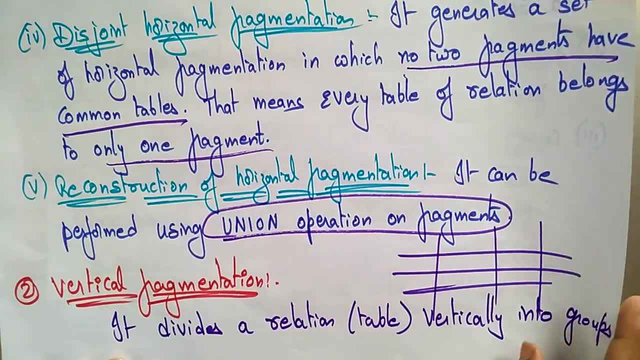 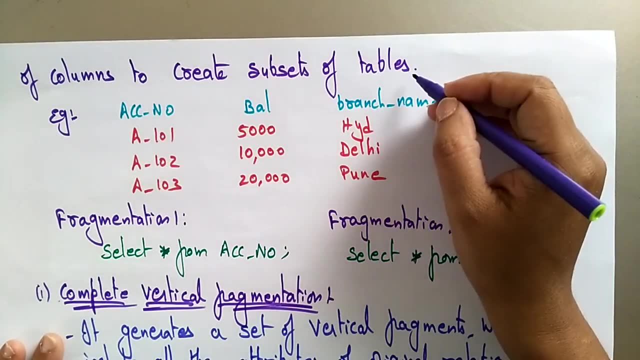 means it devising in the horizontal but in vertical means. it divides the table in vertically and vertically. it divides the relation table vertically into two groups, into groups of columns to create a subset of table. so here you can take account, number, balance, branch, name. so it is divided into vertically. so I want to